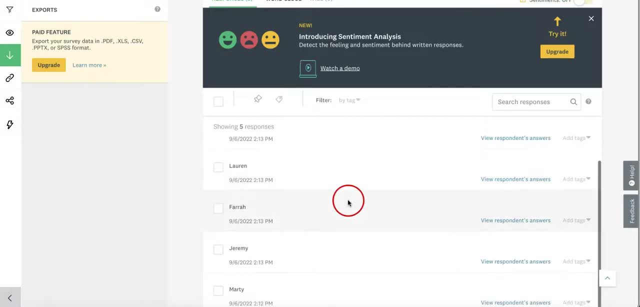 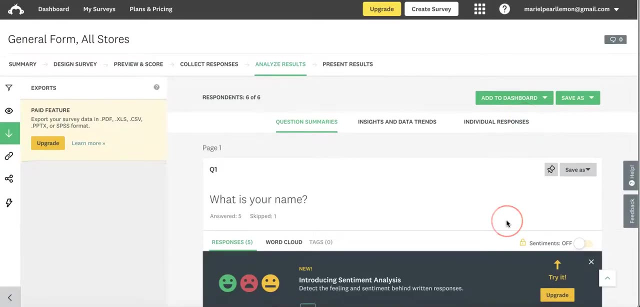 Since we had our identifiable information here. so a lot of the names are here And from here you can actually view each respondent's individual responses One by one. Now, in order to view individual responses, we have two ways of doing this. 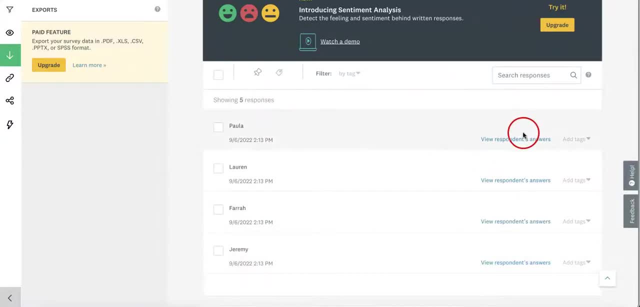 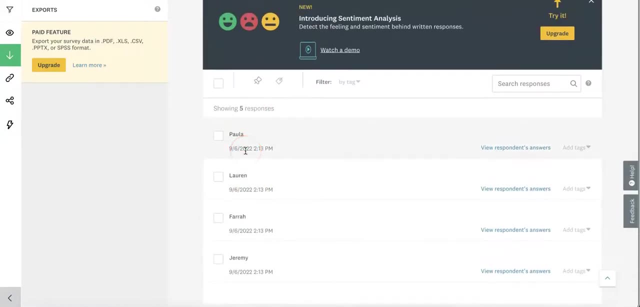 First off, you can do so by looking down right here. You can look at this first section where we have each respondent's name down, So each one refers to a specific overall set of answers And on the right hand side of each name you're going to see that you can actually view the respondent's individual answers. 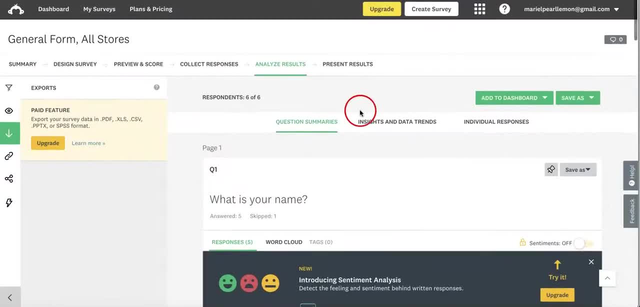 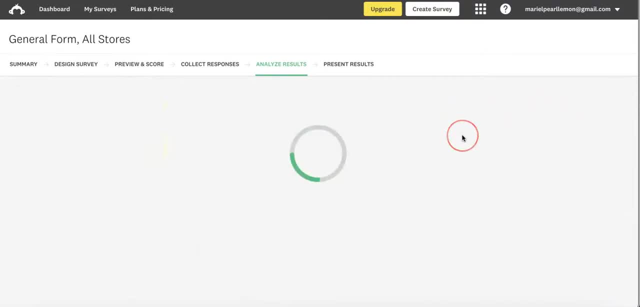 Another way to navigate to the same page Is to head over to the upper right corner here You can see, as we were on the question summaries page, you can also hit the individual responses button right here. So I've just clicked it so we can show you guys what it would look like. 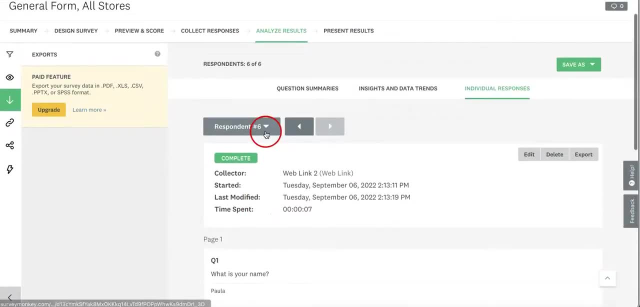 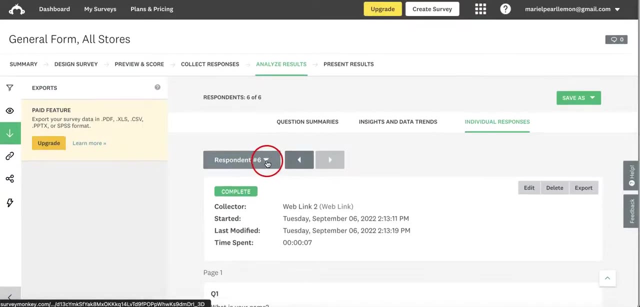 And from here, it's going to show you what each respondent has been answering. Now, in order to navigate between individual respondents, you're going to notice that each respondent is identified by a number, which could be used as a sort of identification number or ID, in this case. 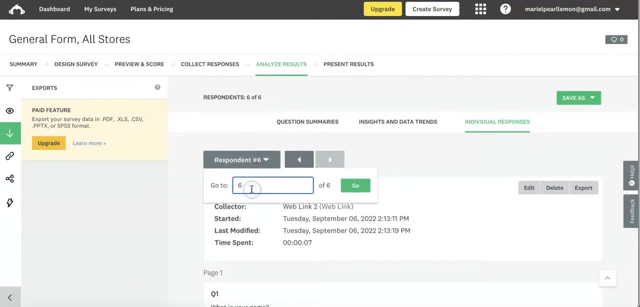 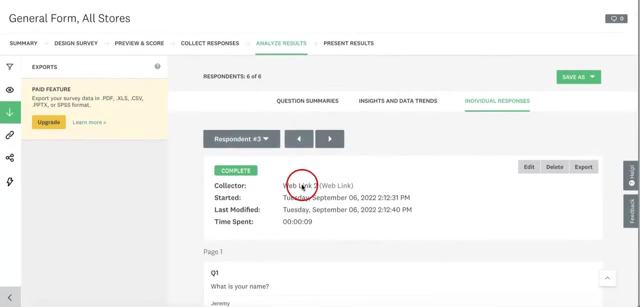 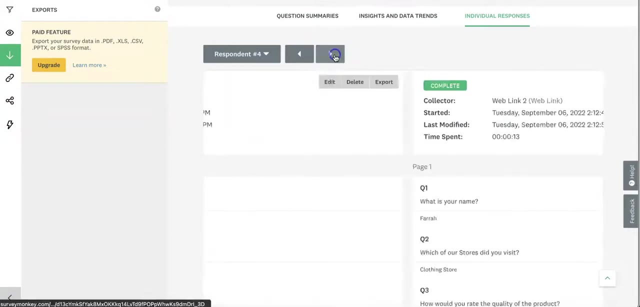 And since you only have six, you can actually go through- Oh my gosh- Most any of them by just simply typing which respondent number they are currently under. You can also just hit back and forth the back page or the next page to see each other set of answers from another respondent. 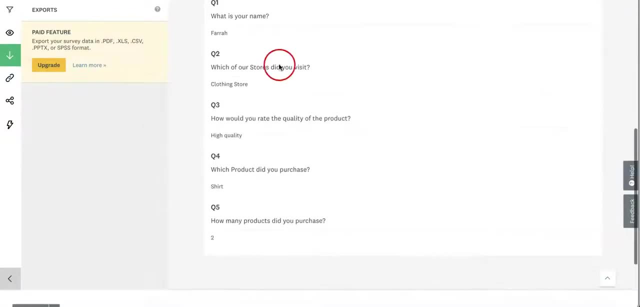 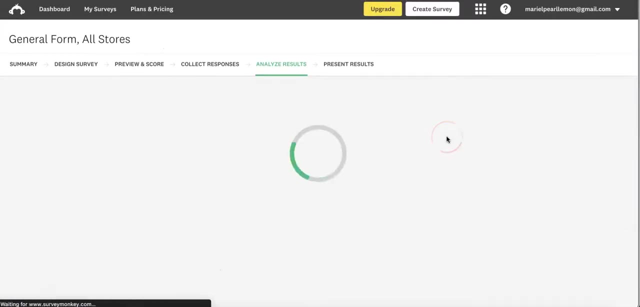 So navigating is actually really easy for anyone who might be wanting to view the individual answers of each respondent. Lastly, we just wanted to go through the insight and data trends so that you guys would be able to see what this would look like and what exactly. 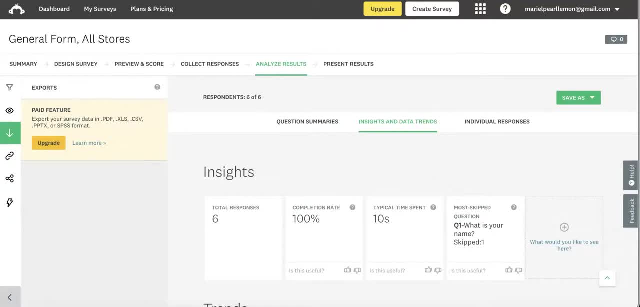 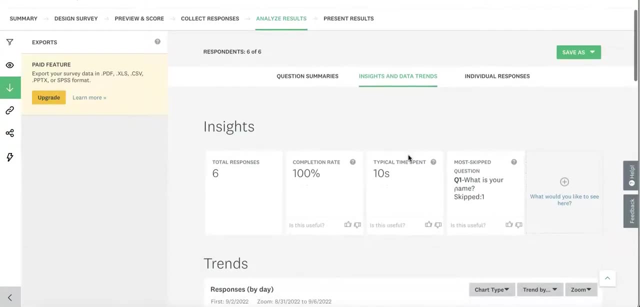 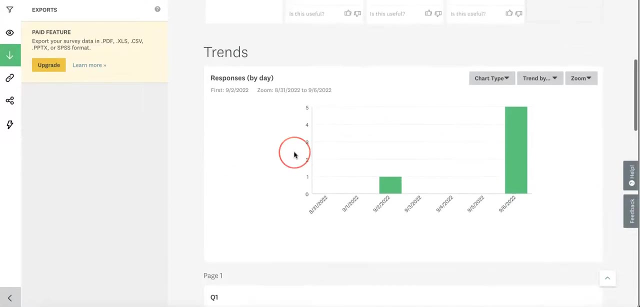 SurveyMonkey allows you to see, or what information or statistics or insights that they actually have already set up for you automatically Now, currently, we're on the free account, So, even though you might not have the paid feature, you can actually see all of this information on any of your forms as of now. 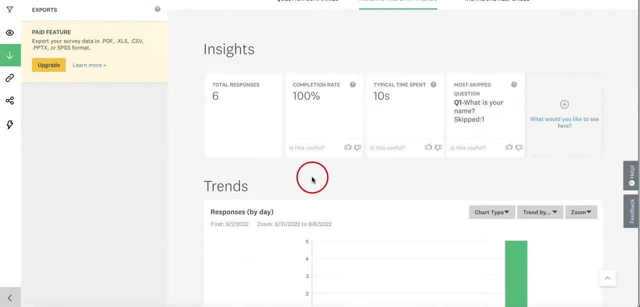 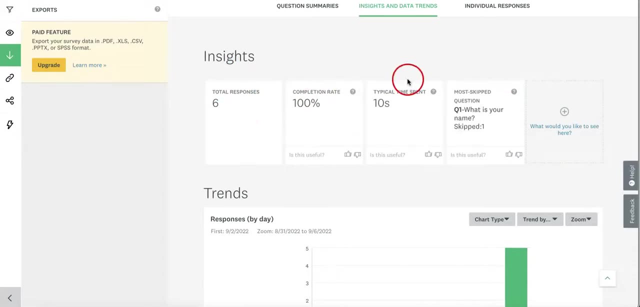 Okay, So you're going to see on the insight section how many total responses you've got, the completion rate, which is 100%, which is really good for us. Okay, You'll also see the typical time spent on each survey, So you can see it's a very quick one too. 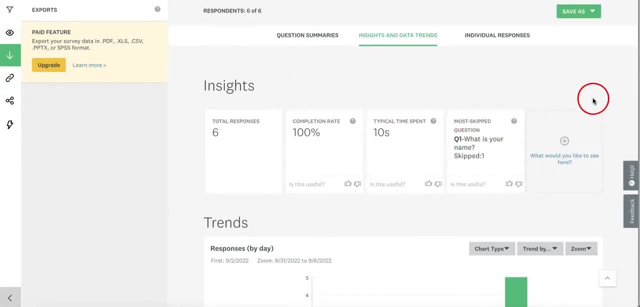 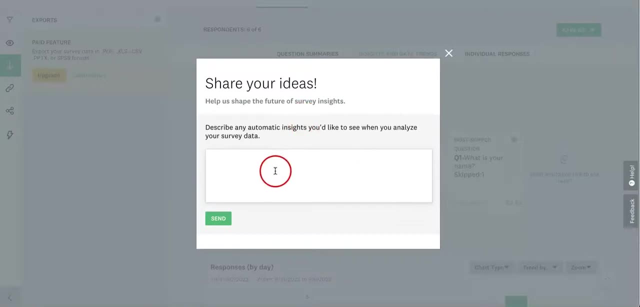 And, lastly, you're also going to see the most skipped question. Now, these are just the generic insights that SurveyMonkey provides. You can actually add more if you want to see what other automatic insights you'd like to see when you analyze your survey data. 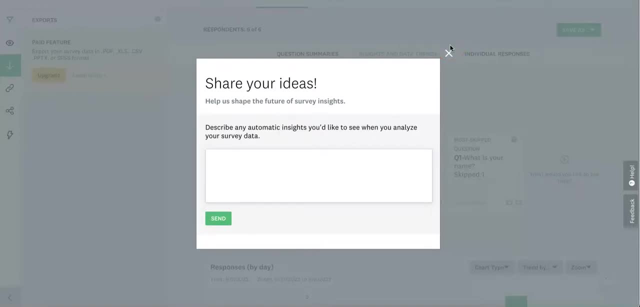 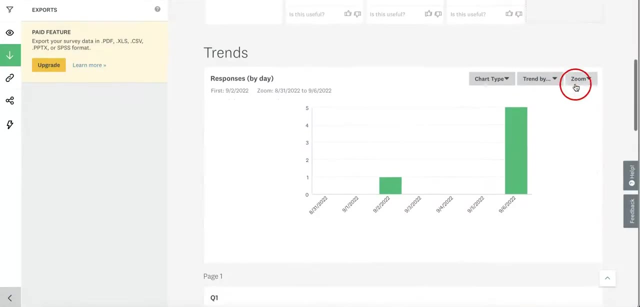 But this does not actually add anything to your analysis. This is just more so of a suggestion that you might send over to SurveyMonkey and see they might actually respond and help you with that. Next, you're also going to see that we have the trends page. 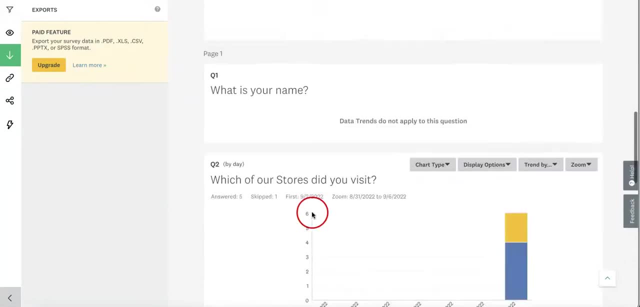 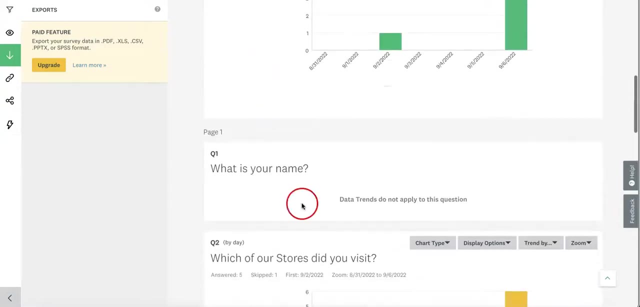 meaning that we can see how many responses you've been getting by day. You can also see the statistics on certain questions, depending on what kind of answers they give. So for the name questions or the single text box questions, we're not going to see a lot of this here. 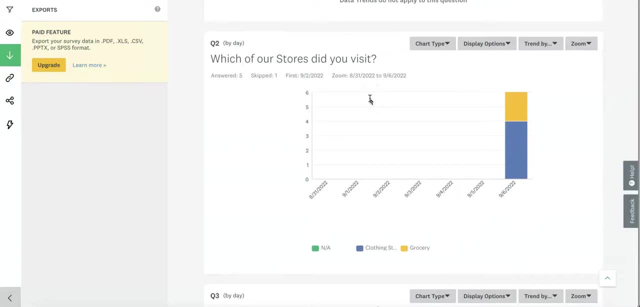 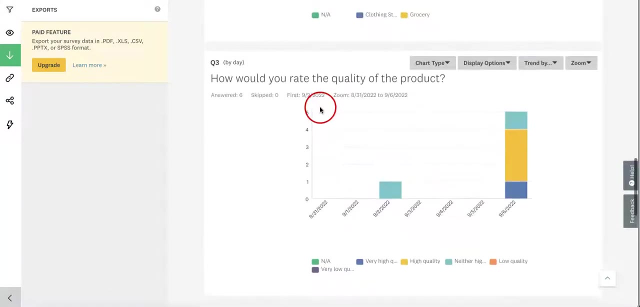 You're more likely to see this in the more close ended questions, such as the multiple choice questions or the checkbox questions. So here we can see which of our surveys were actually most visited. We can also see how people are currently grading our product according to date. 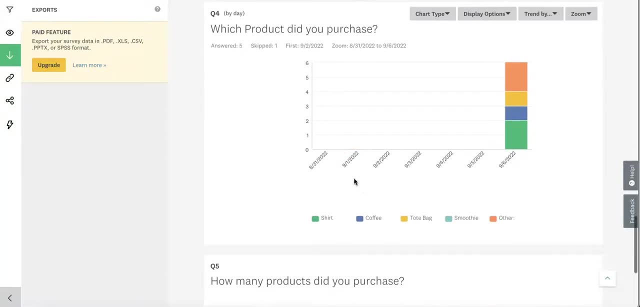 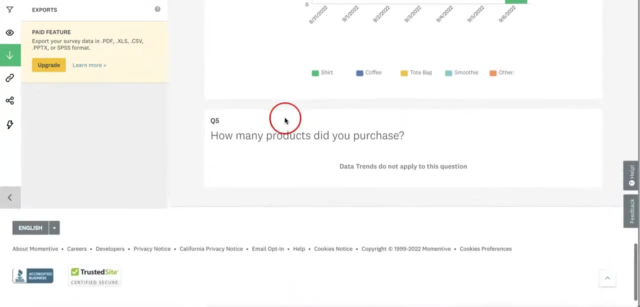 We can also see which products are being purchased according to date, which is also interesting, seeing as most of our products are being purchased on a one day only. And that's about it for our form. Okay, so that was just the basics on how the analyze results page works.